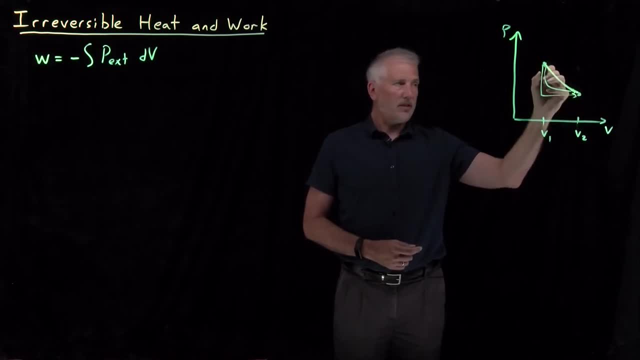 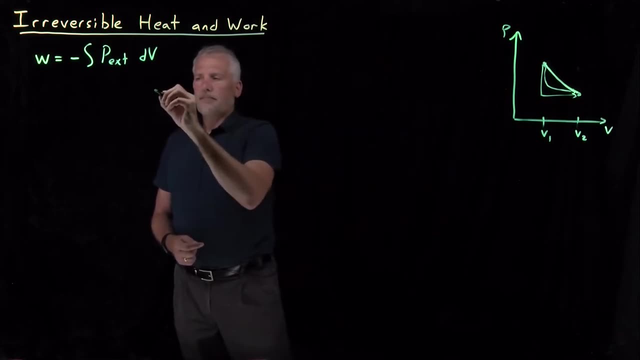 case. The only reversible isothermal case is this upper line. There's a lot of different irreversible paths And what we've seen so far is that 0.3 numerically for the cases. we've seen so far the work done. when we do the process. 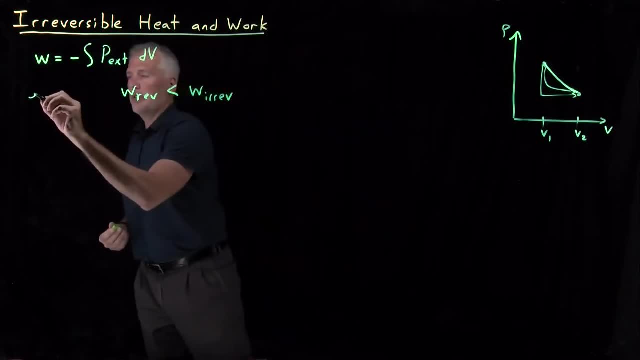 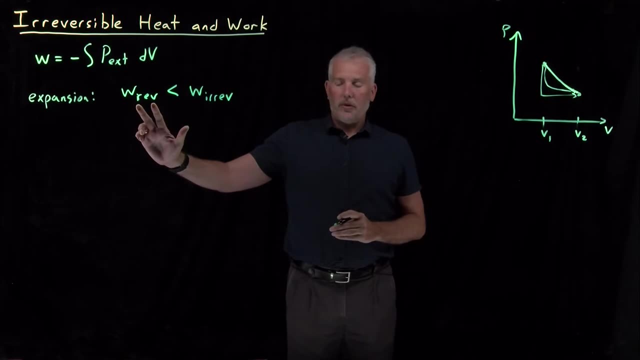 reversibly for an expansion of a gas. So let me make sure this is for an expansion. The work done in the reversible case has been less than the work done for the irreversible case. In particular the negative: when a gas is expanding, the work is negative. 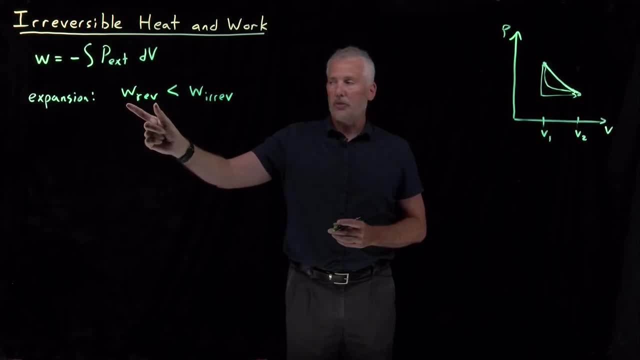 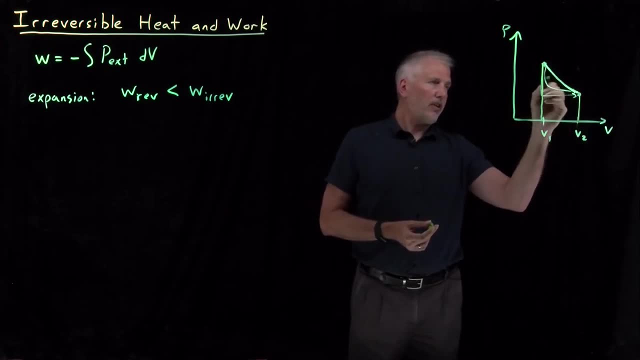 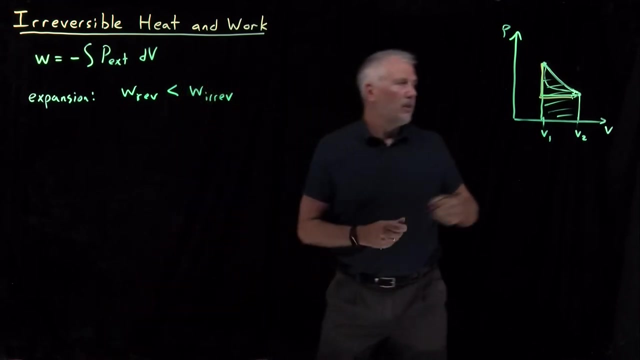 So that negative number is a larger negative number for the reversible expansion than for the irreversible expansion. And the reason that's true is that if we calculate the area under these curves, the area under the upper curve does a greater area of expansion 0 these curves 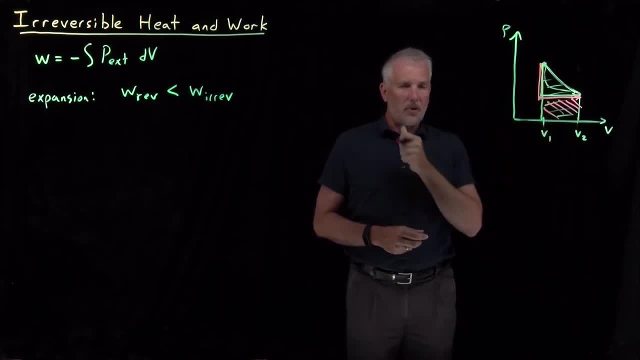 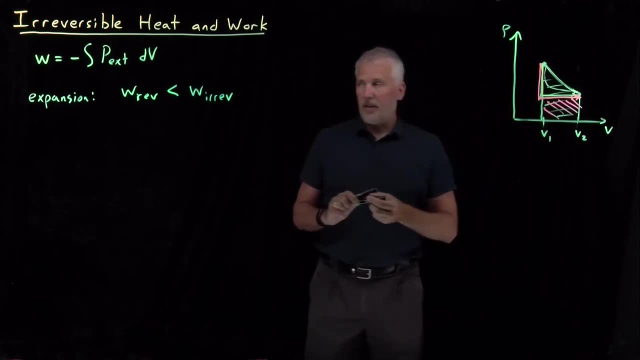 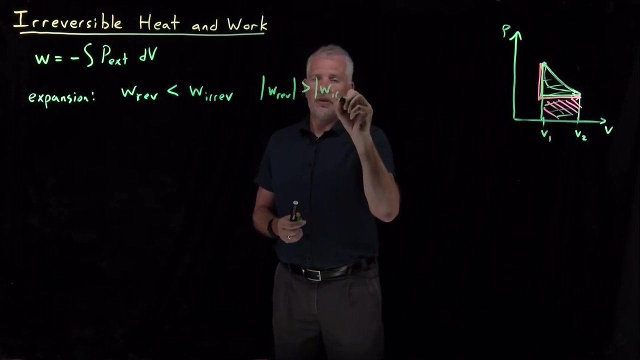 D, smaller area than the area under the upper green curve. So that means whatever irreversible line I draw, the size of that area, the magnitude of the reversible work is going to be a larger magnitude than under the irreversible curve And because those values are negative, the larger 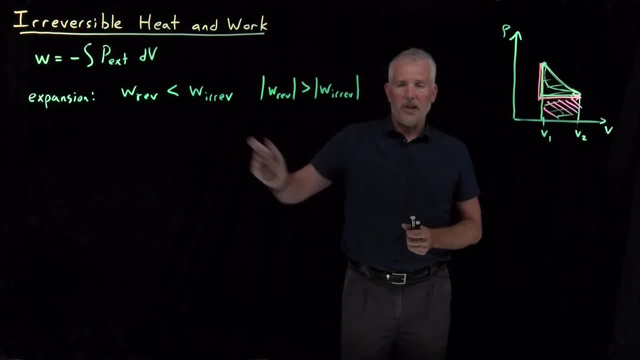 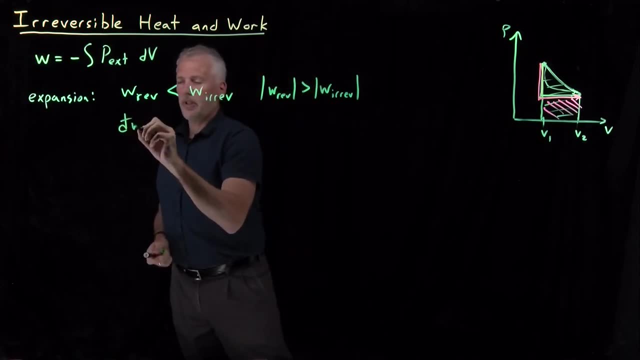 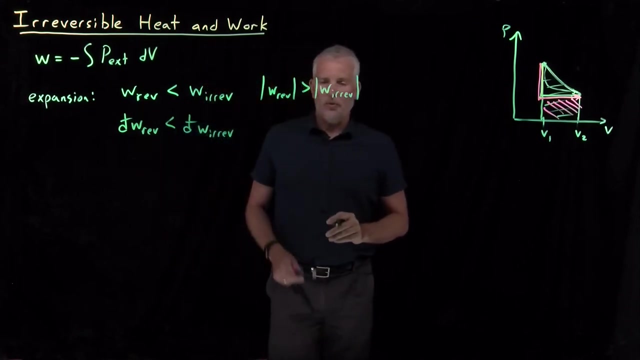 negative number is smaller than the smaller negative number. And the other way we can think about it, that is, even if I were making large changes for a small, infinitesimally small change, the tiny amount of work that I do for a reversible process is smaller, meaning more negative. 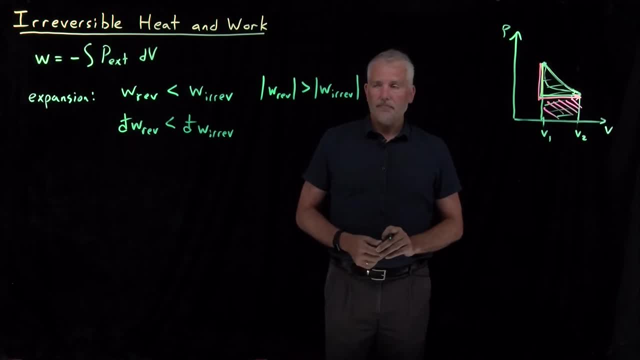 than the amount of work I do for an irreversible process, So that all holds true for an expansion. Easiest way to think about that is perhaps with these graphical curves in the area under this curve with a negative sign in front of it. We can also ask ourselves: 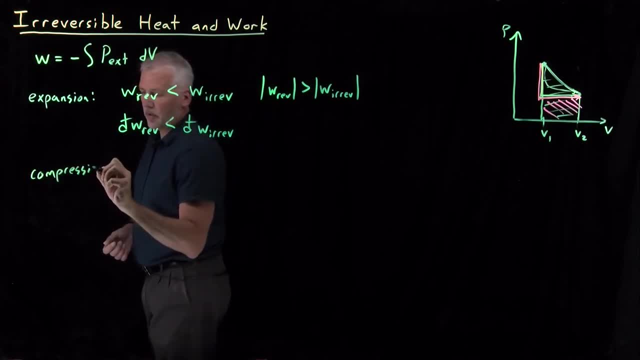 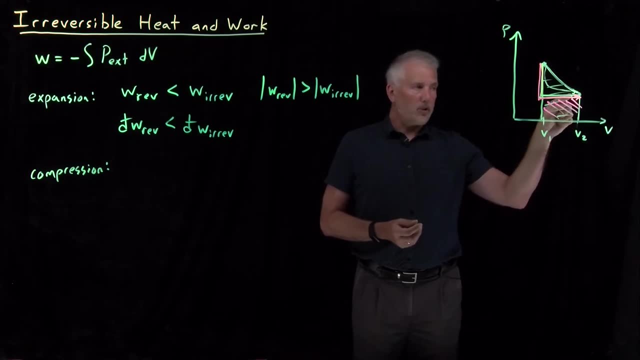 how much of that is still true when we talk about the compression of an ideal gas. So now imagine we're not starting at V1 and going to V2, but we're starting at the large volume and going back to the smaller volume. So the reversible curve is exactly the same When I take a gas and compress. 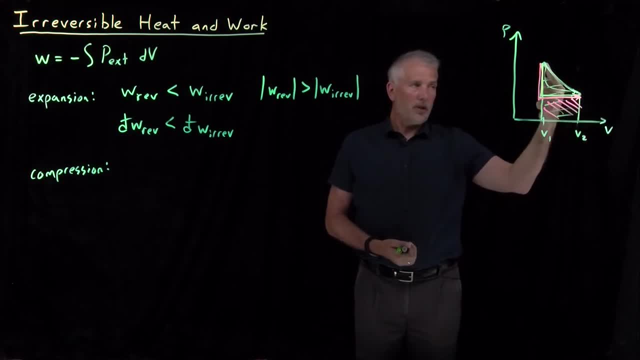 it reversibly, then I, and isothermally then I'll move along this curve right here. If I were to compress it irreversibly, the way I'd have to do that is not by releasing the pressure but by letting the gas spontaneously expand against that release pressure To compress the gas. 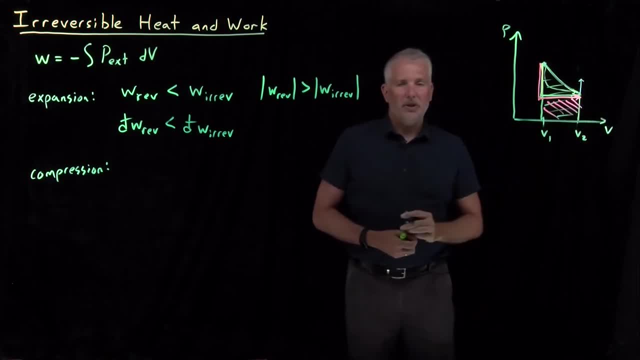 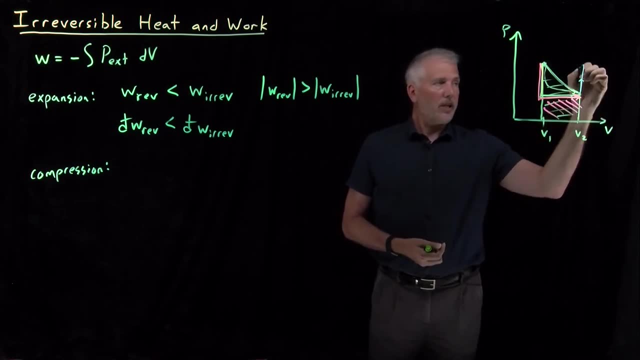 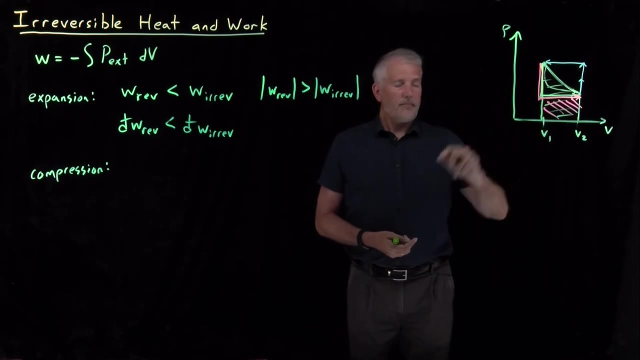 irreversibly. first, what I have to do is increase the pressure too much and then let the gas compress as a result. So a very irreversible compression would be. go ahead and increase the pressure all the way to the final pressure and let the gas compress under that increased. 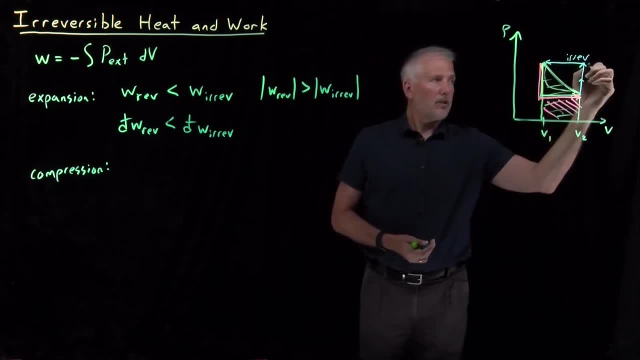 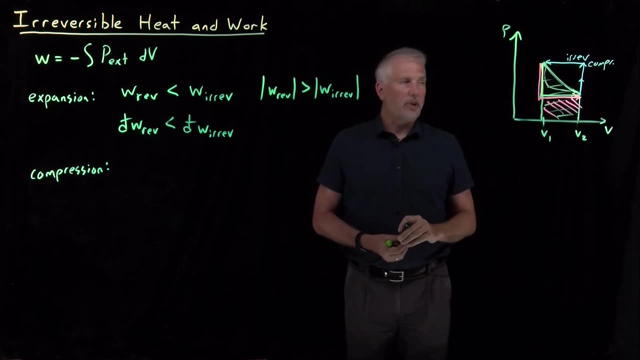 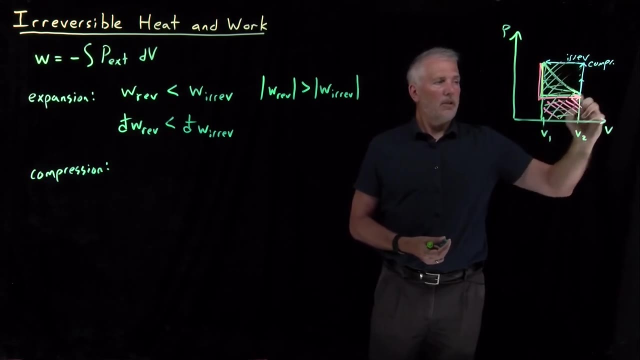 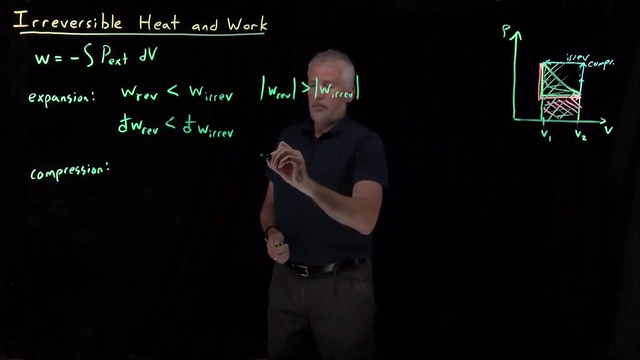 pressure. So this would be an irreversible compression And the green curve here would be a reversible compression. So if we think about the areas under the curves now, now the area under the blue curve is larger than the area under the reversible curve. So what we'd say in that case is from the magnitudes point of view. 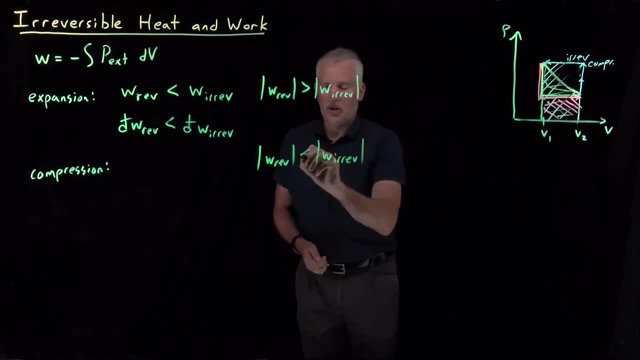 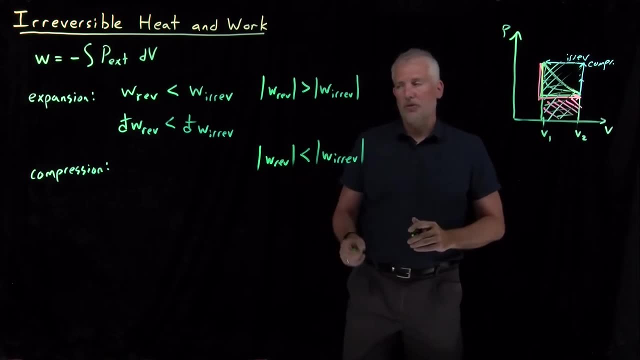 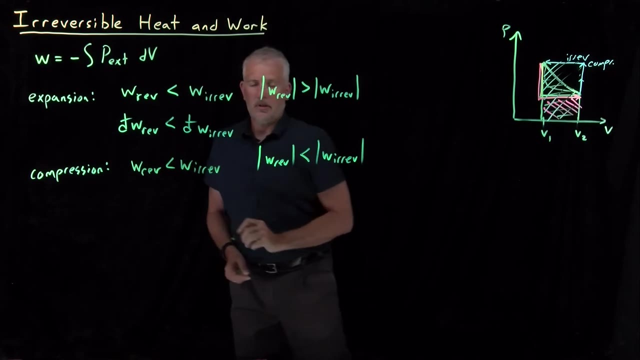 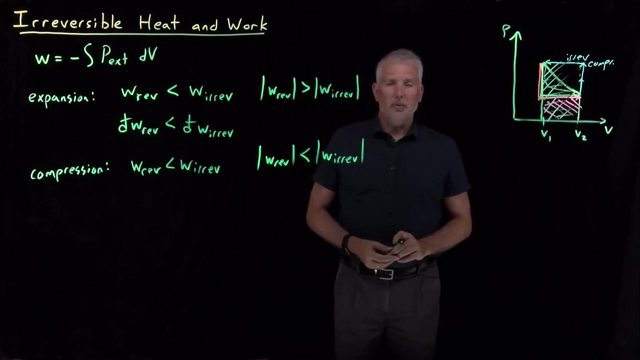 the blue irreversible compression has a larger area than the green reversible compression. But those are positive numbers so it doesn't matter whether I include the magnitudes or not. so if I strip the magnitudes off the absolute value signs the reversible work for compression is less than the irreversible work for 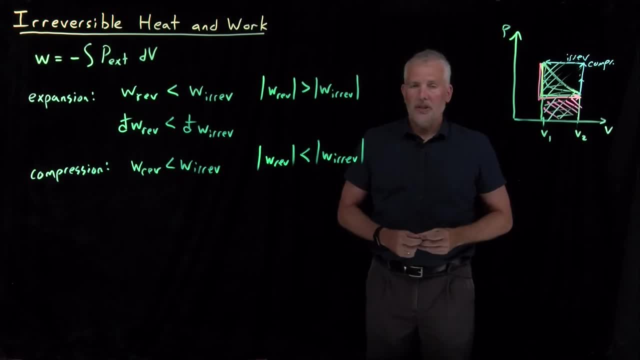 compression, And that makes sense. remember, when we're talking about compression, this is work being done on the gas energy we're supplying into the system in the form of PV work. And when I compress the gas smoothly, gradually, reversibly, I'm applying just as much pressure at every step. 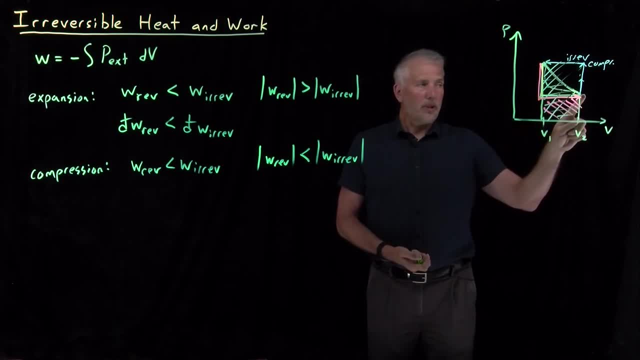 as I need to make the gas compress. If I do an irreversible compression, whether it's via the curve I've drawn or perhaps via some other irreversible curve like that one, I've over pressurized the gas. I've applied too much pressure, so I've done too much work. 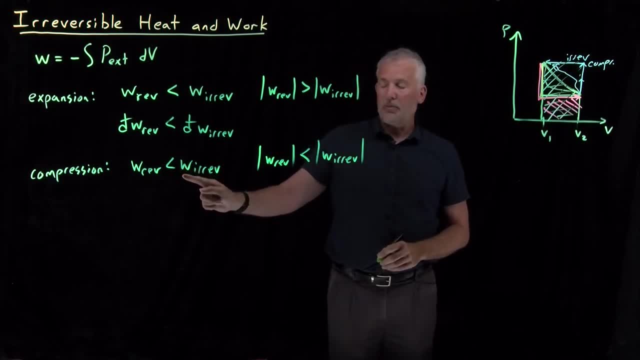 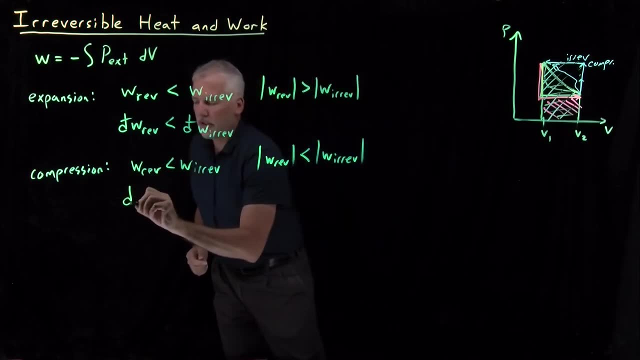 So the work that I've done in the irreversible process to compress the gas is larger than the work that I would have to do if I did it reversibly. So let me go ahead and write down the differential form of that expression: D W- reversible- is always going to be less than D W- irreversible. 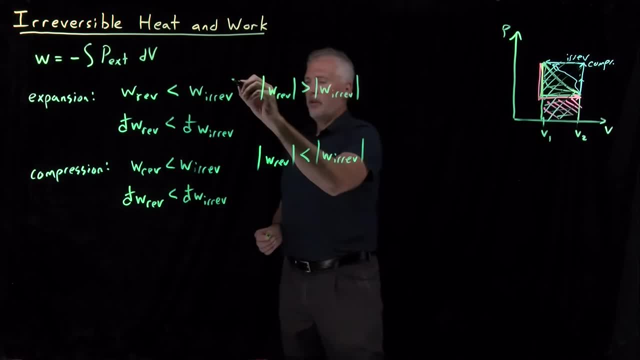 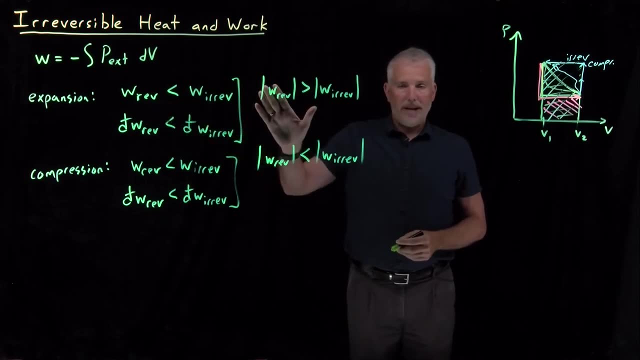 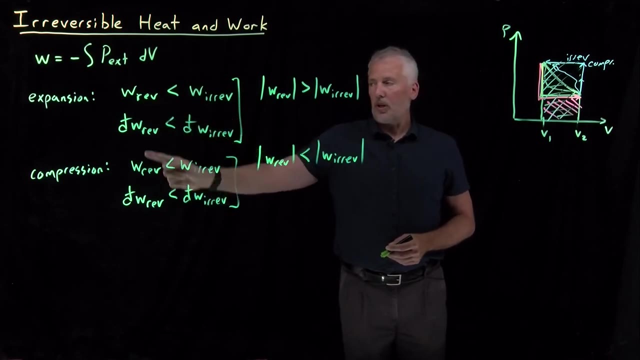 So the convenient thing is, both these two sets of equations tell us the same thing Numerically, without worrying about magnitudes, just the value of the numbers, including positive and negative signs. reversible work is always less than irreversible work, regardless of whether we're doing an. expansion or not. So that's the difference between the two sets of equations. So let me go ahead and write down the differential form of that expression: D W- irreversible- is always going to be less than D W- irreversible. So that's the difference between the two sets of equations. 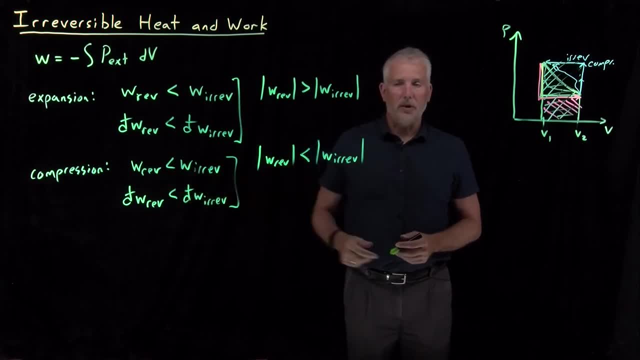 So that's the difference between the two sets of equations. So that's the difference between the two sets of equations. So reversible work is less than irreversible work. The physical interpretation of that statement means: when a gas is expanding, when I'm letting it expand against some external pressure. 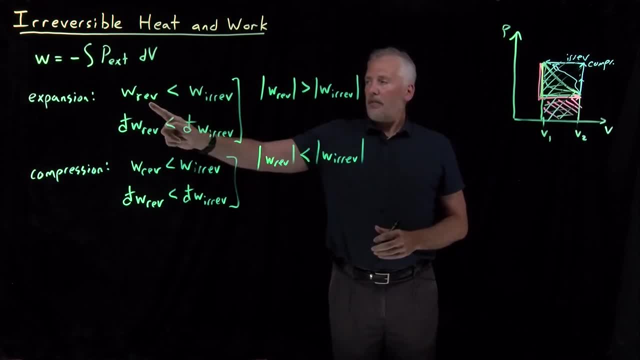 then the value of the work is more negative, meaning it's a larger magnitude. So I can get the most work possible out of the gas If I'm allowing the gas to expand and the gas is doing work and I'm using that work to do something useful. 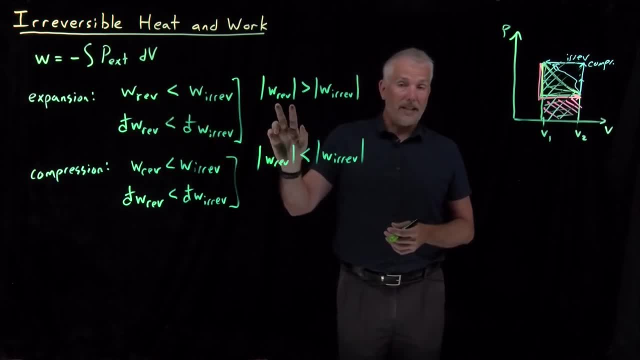 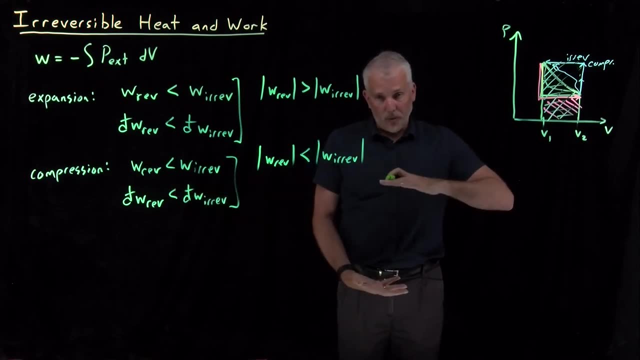 I get the most work possible out of the gas. I get the most possible work out of the gas, the largest magnitude of work out of the gas, when I allow it to expand reversibly. On the other hand, for a compression, if I'm the one doing the work on the gas. 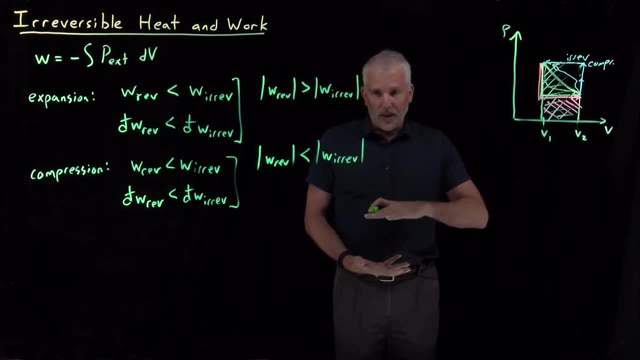 then when I do the gas reversibly, I get to do the least amount of work possible on the gas when I do it reversibly. So in either case, reversible is good for us. We get a lot of work out of a gas when it expands reversibly. 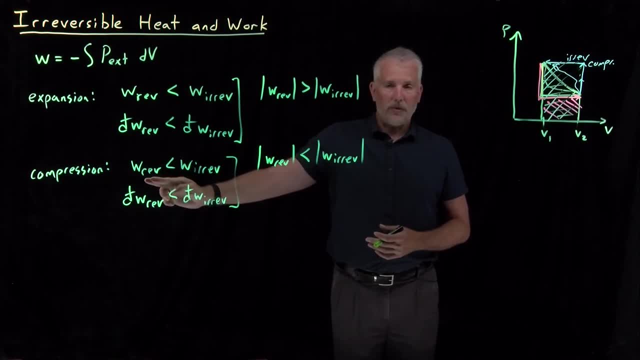 We don't have to do as much work when we compress it reversibly. So that's one way of remembering these inequalities. So that's one way of remembering these inequalities, to remember that we, the external surroundings, win in the reversible process. 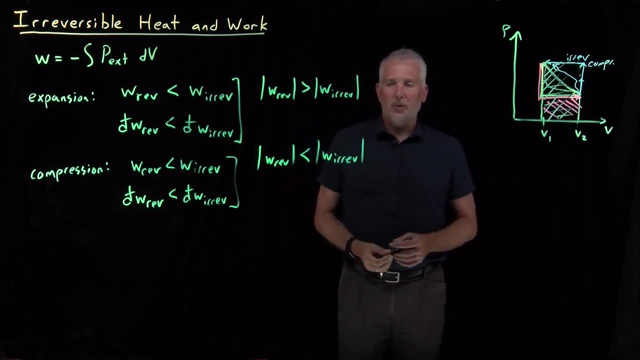 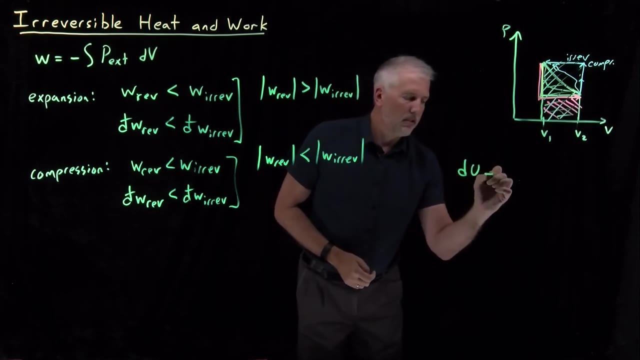 either getting a lot of work out of the gas or doing as little as possible to the gas. So the next thing to talk about, now that we have these inequalities is: what's the equivalent statement? not about work, but about heat. And we can, because we know the first law. 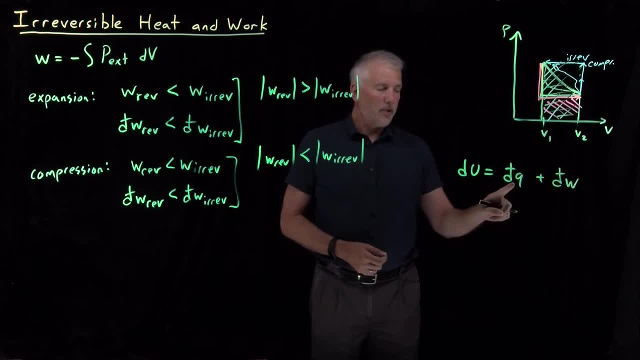 there's a connection between the two. There's a connection between heat and work, Remembering that heat and work are path functions. These are inexact differentials, which means they're path functions. U is a state function. It's an exact differential. 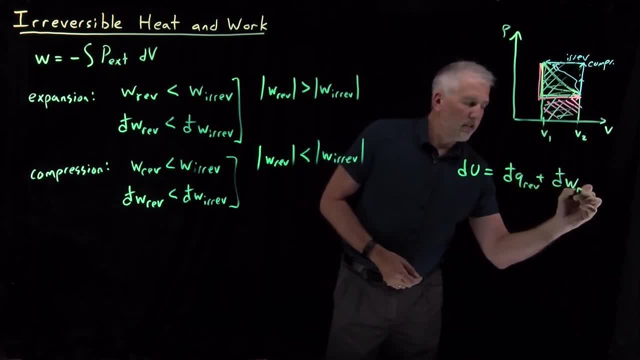 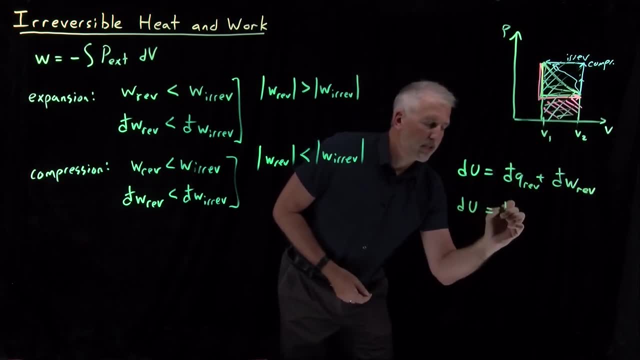 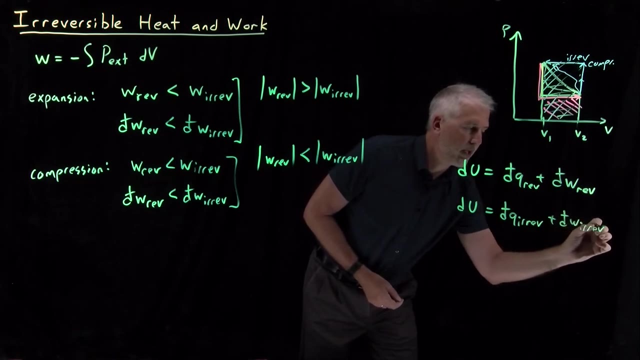 So it doesn't matter whether I write for a reversible process. D? U is D Q plus D W, Also true for an irreversible process. First law is always true. So if I think about again some reversible path and some irreversible path, du is the same. 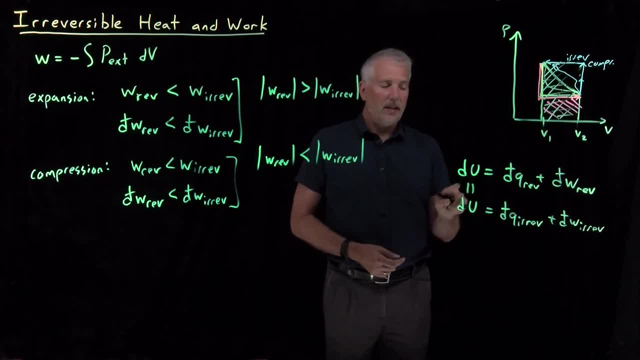 Remember, du is a state function, so it doesn't matter what path I take, du is the same, no matter how I get from state one to state two, so that du is either equal to this reversible dq plus a reversible work or irreversible dq plus the corresponding irreversible work. 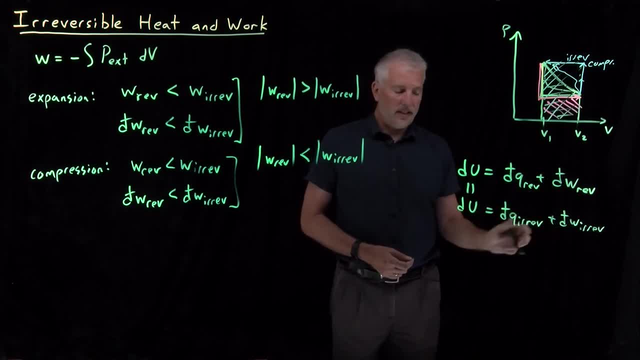 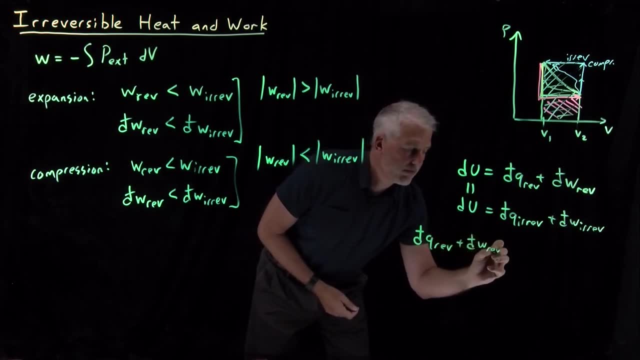 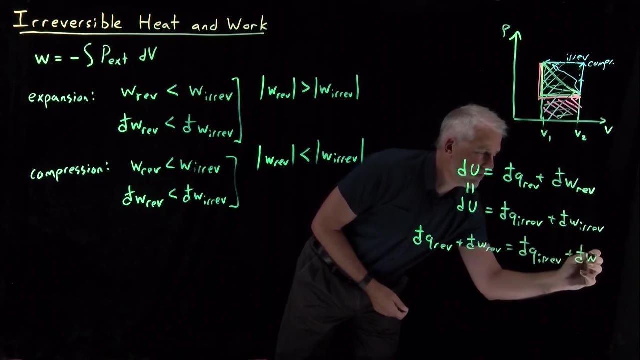 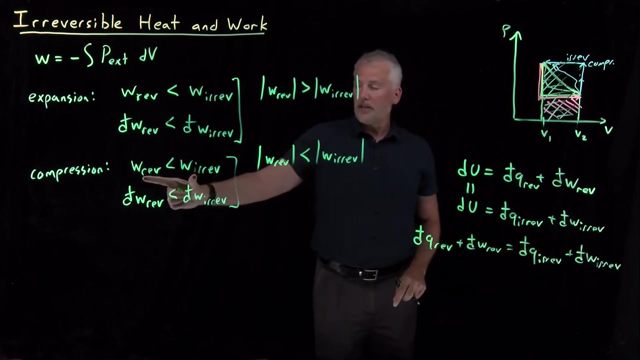 So if I set these two right-hand sides equal to each other, so I can say dq- reversible and dw- reversible- must be equal to the same sum for any irreversible path that I choose. I already know something about the relative size of where the reversible and irreversible works. 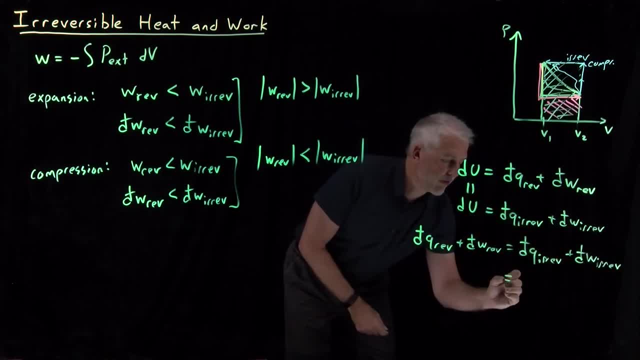 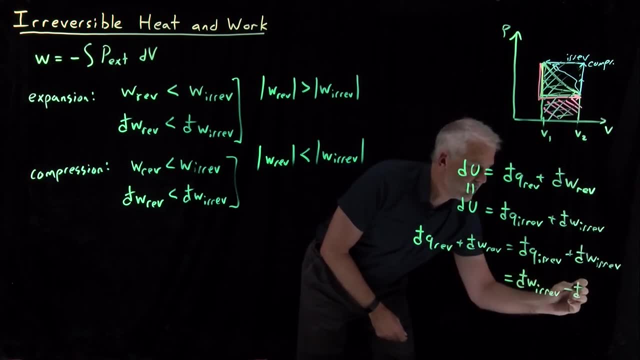 so if I get these two dws on the same side, let's put those both on the right, so I'll leave dw irreversible on the right and I'll bring dw reversible over with a negative sign And I'll get the qs both over to the left. 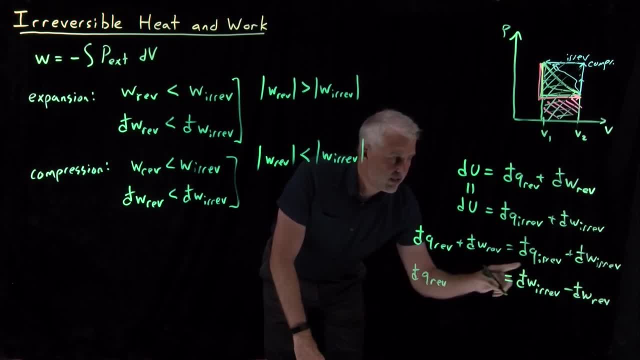 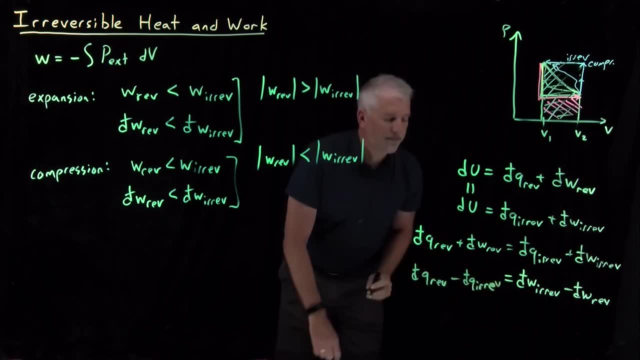 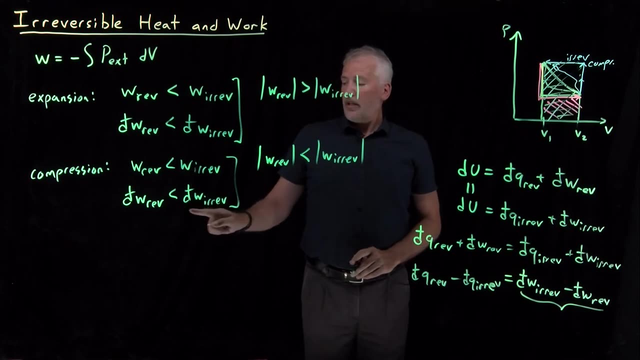 so in that case I've got dq reversible and I'll bring dq irreversible over with a negative sign. And now we know from the reversible work inequality: the reversible work is always larger than sorry. the irreversible work is always larger than the reversible work. 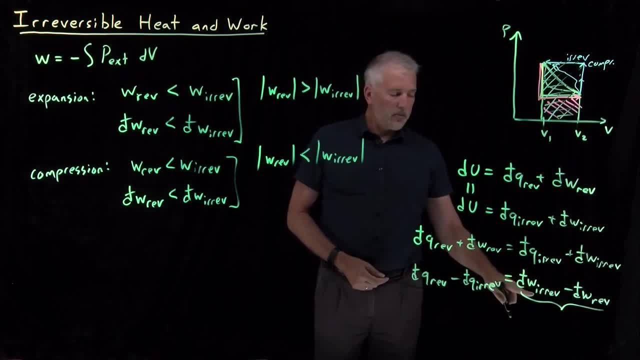 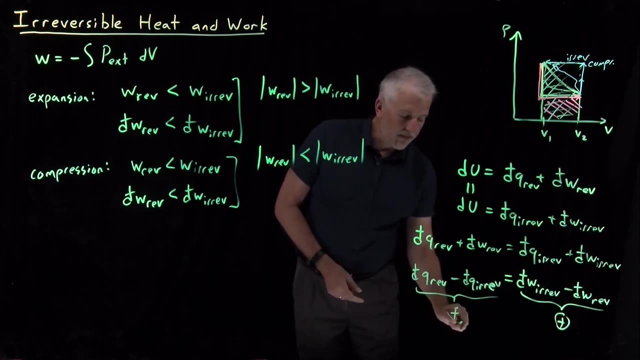 regardless of what they were doing: an expansion or a compression. so irreversible is larger than reversible. so this difference is a positive number. so whatever that difference is, it's the same as on the right hand side, as on the left hand side. so this difference on the left also must be positive and in 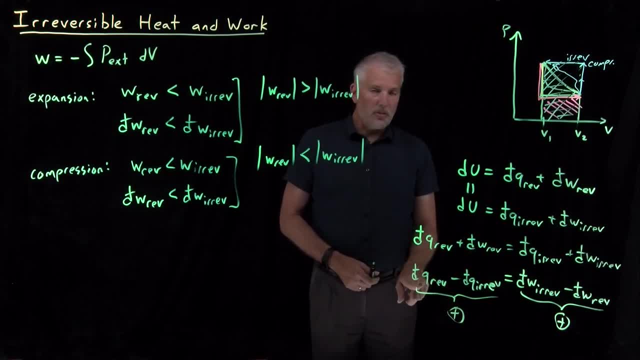 particular, the same positive number. so what that means is the reversible heat minus the irreversible heat is always going to give me a positive number. so what that means is the corresponding version of this statement for the heat is that DQ reversible is always going to be bigger than DQ irreversible, and